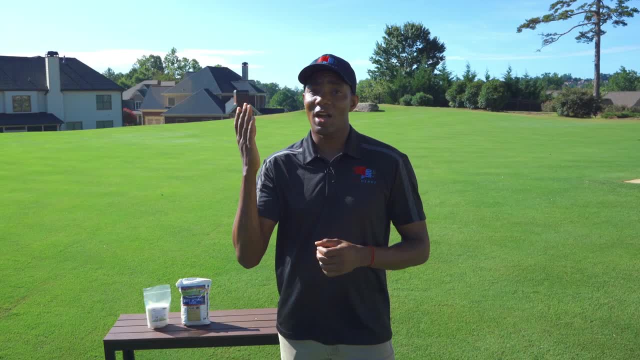 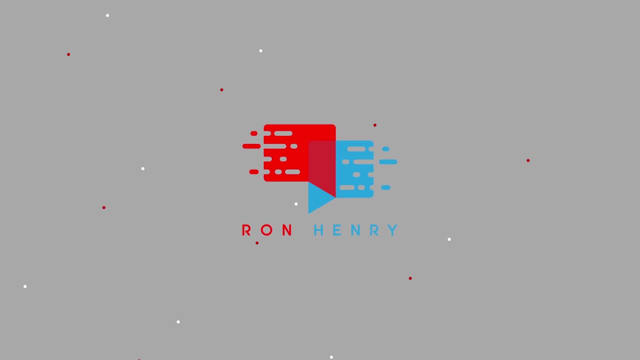 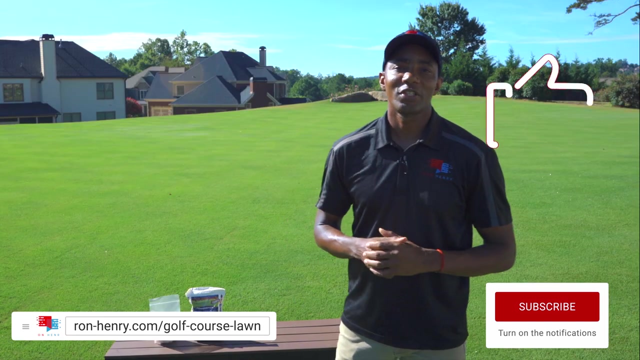 So you just got your soil test results back and perhaps your pH is too high or too low. Let's talk about options for fixing that. Hello YouTube, Welcome to Project Golf Course Lawn, Season 5.. So you just got your soil test results back and perhaps your pH levels are a little bit out of whack. If they were super high, the results. 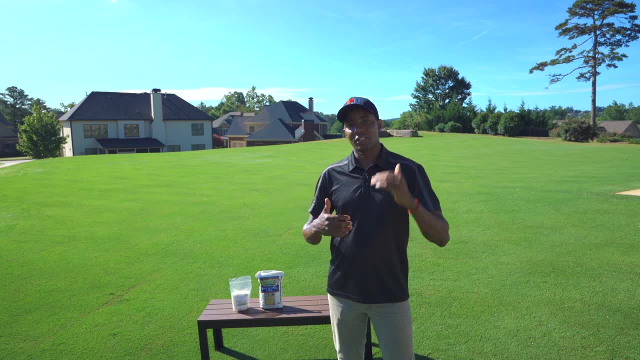 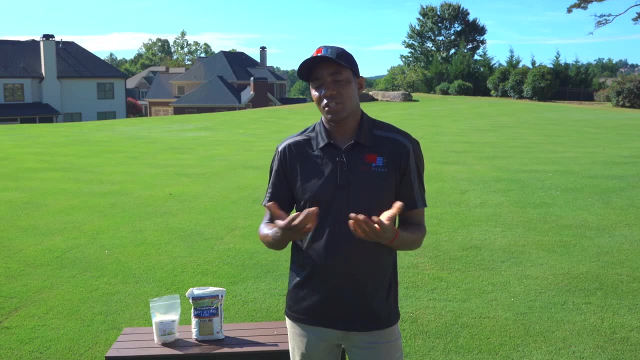 are going to say that your soil is too alkaline, and if they are excessively low, your results will say something like your soil is too acidic. So why is that important? Why is pH important at all? Why should we care about it? Well, most plants- and grass is no different- have a certain area a certain range that they do well. as far as nutrient uptake based on soil pH, When your soil pH gets too low, the soil begins to get more acidic and again that hampers nutrient uptake. In the case of soil pH getting too low, it also begins to 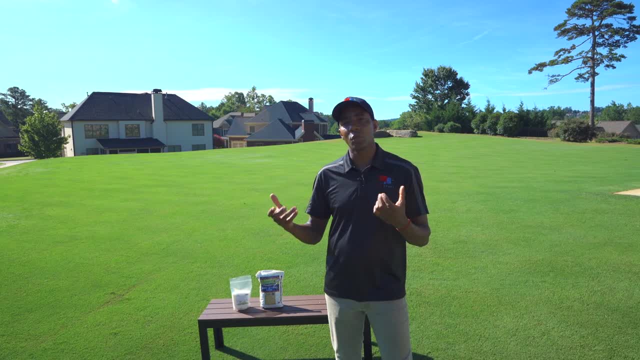 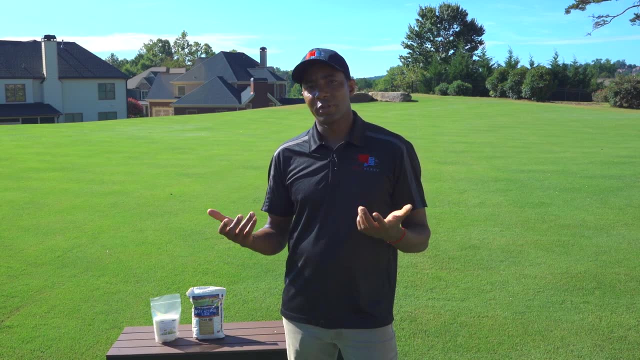 allow certain elements that normally would not be available to the plant to become available. that creates problems. So a good example: if your soil pH is excessively low, aluminum- which is not something that your soil really needs- becomes available, and that can do things like stunt root. growth, which in turn hurts nutrient uptake. When your soil pH is too high, an element called molybdenum becomes available, and that is just downright toxic. So in addition to you not getting absorbed by your fertilizers, the soil actually becomes toxic for your grasses. Other micronutrients: 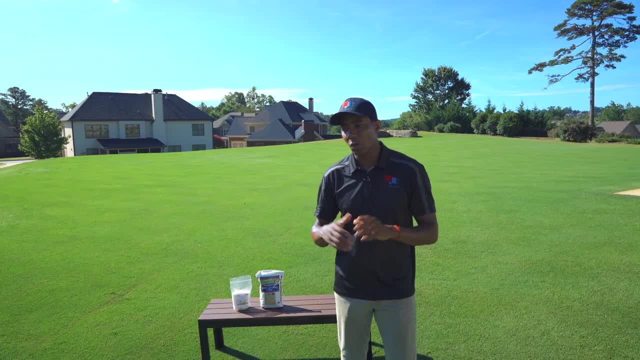 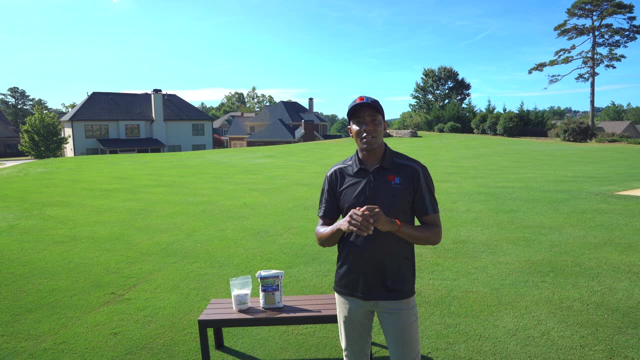 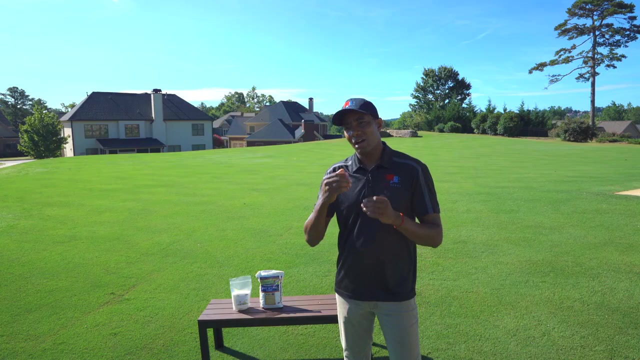 like iron, just aren't absorbed as well. So as far as the sweet spot for most grasses, we're talking about Bermuda. in general, Bermuda likes a soil pH somewhere between 5.8 and 7.2, anywhere within that range you're going to be okay. Low to mid-6s is perhaps a. 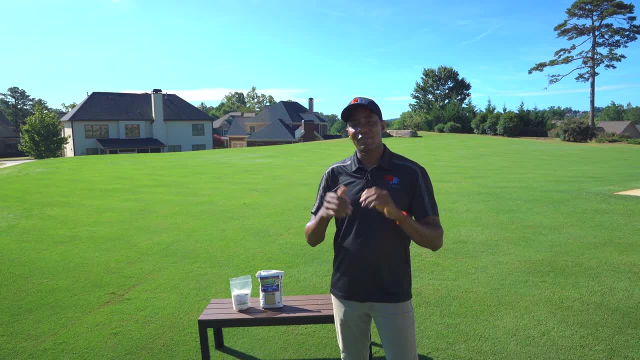 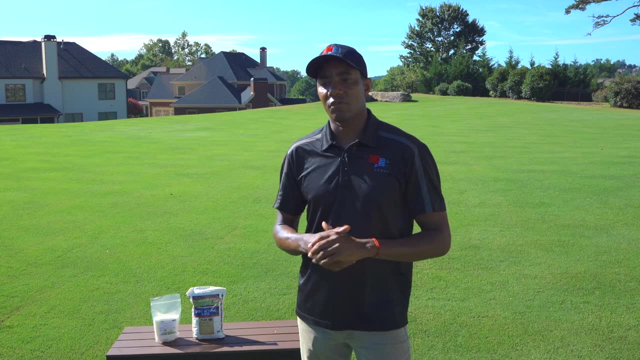 sweet spot. but as long as you're within that range, you're going to be okay. between six and seven you're gonna be all right. so what happens if your ph is incredibly low? like, what do you do to to fix that? because this is a question i've gotten from you guys, so forget to. 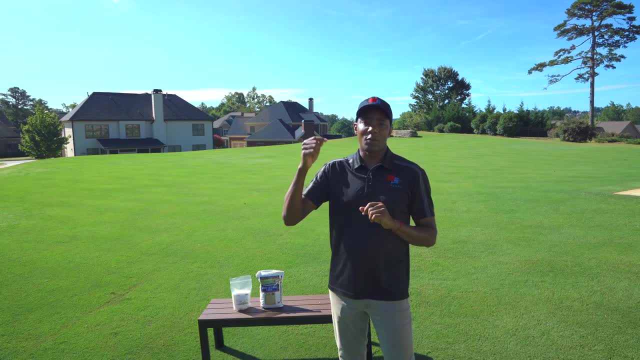 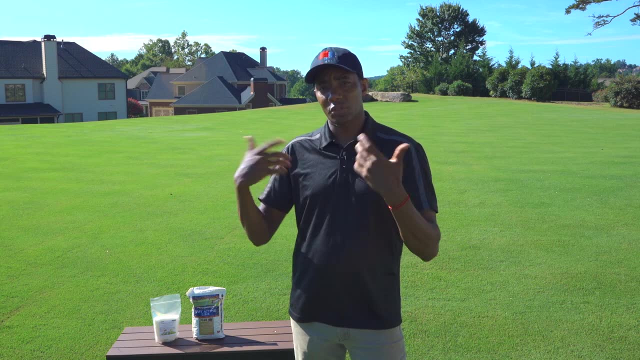 make a video on it. so the way to to think about this is: if your ph is low, the the, what you're going to want to do is you're going to add lime to the lawn. so low, add lime. that's what you're going to use to to raise uh soil ph and if your ph is excessively high, you're going to use you want. 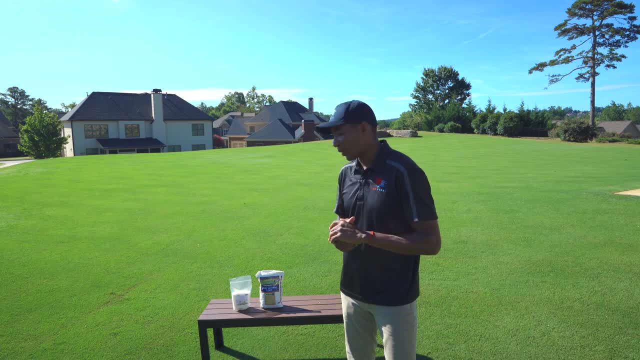 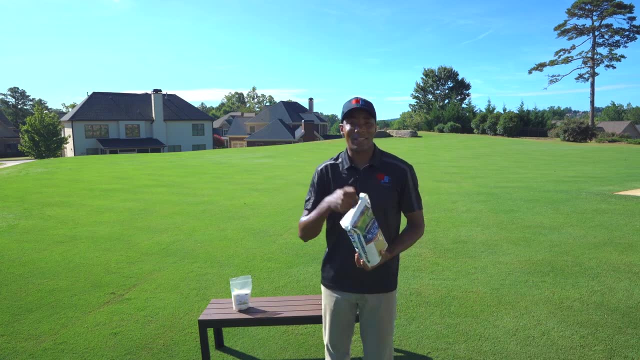 to apply some kind of a sulfur, the. the sulfur i'm going to show here is an ammonium sulfate that's going to help to lower your soil ph. so again, i don't really have a a thing to remember for high ph. just remember, if it's not um, if it's high, the other one, that's not lime. as far as 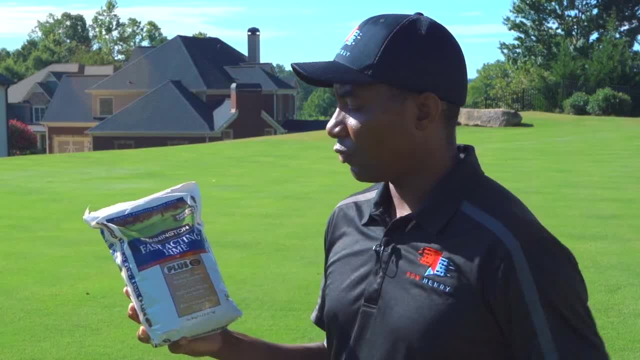 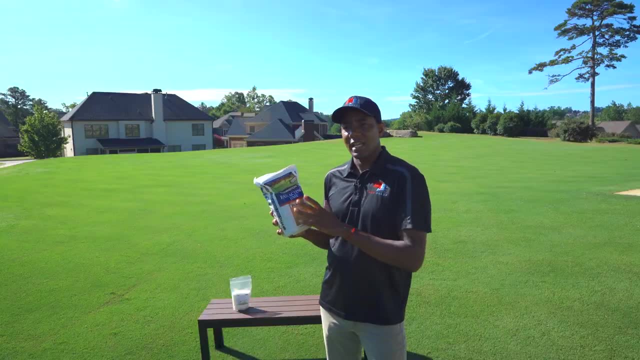 recommendations for a good lime product. i really like this one from pennington. it's a it's a fast acting product. it once you apply it and you water the lawn heavily, it breaks down relatively quickly so it can be used by the soil. so this is a great one. you can probably find this one at your home depot, your. 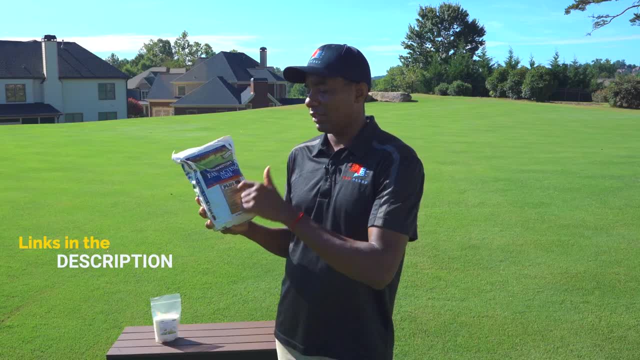 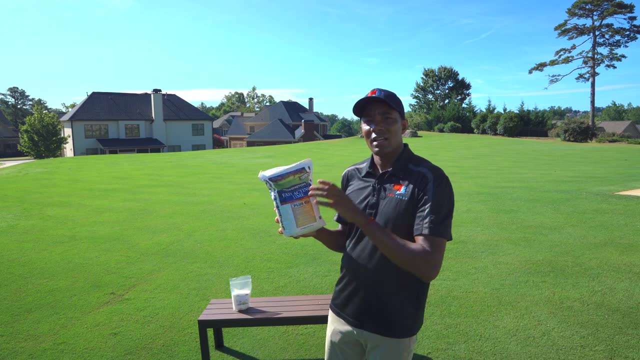 lows your big box stores. and if you can't find it there, i'll also have a link for this in the description where you can pick this up on amazon. the way this goes down is: this is a six pound bag. six pounds covers a thousand square feet, so depending on the size of your lawn, 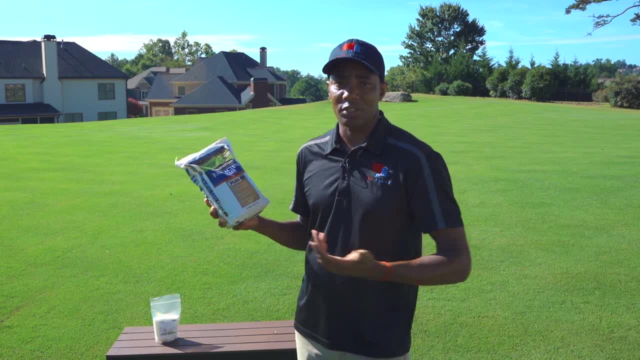 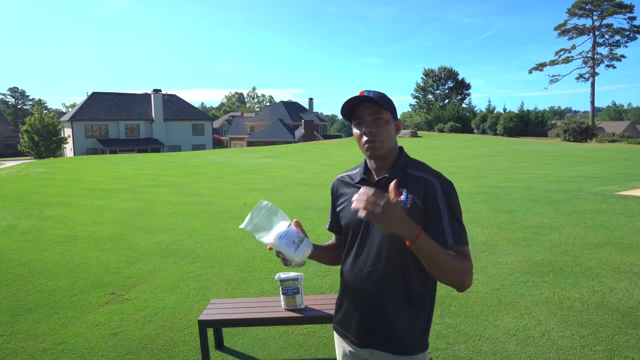 you'll know how much of this you need to get. i didn't get a huge bag because i don't really need to adjust the ph of my lawn, but i just wanted to have the product to be able to show you guys as far as what i recommend you use, as far as a lime for lowering ph. 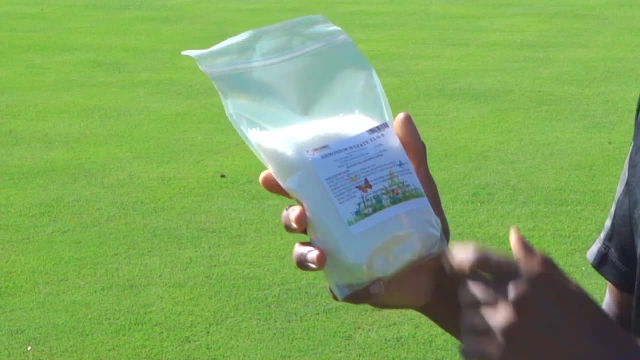 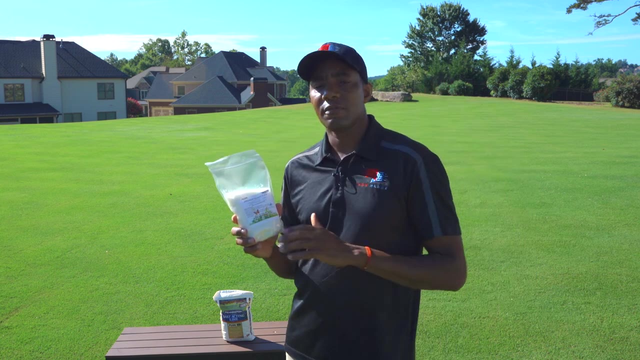 the product i'm going to recommend is an ammonium sulfate from greenway. this has got 24 sulfur in it, and the one thing i've seen- that's that's fairly common- is that most of the sulfate products also contain nitrogen. so in the case of this one from greenway, you've got 21 nitrogen as 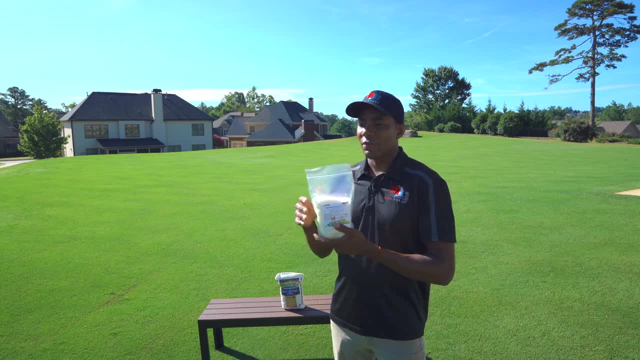 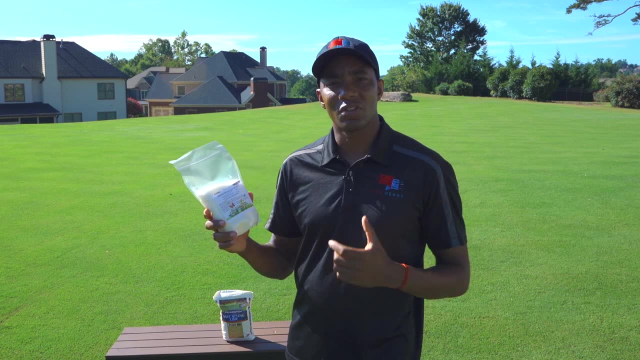 well. so you know, kind of take that into account. you know, if you're due for a fertilization, perhaps use a fertilizer that's a little bit lower in nitrogen, since you're going to be applying this to the lawn to try and lower that soil ph level. so you canannon put one in the garden. so you're going. 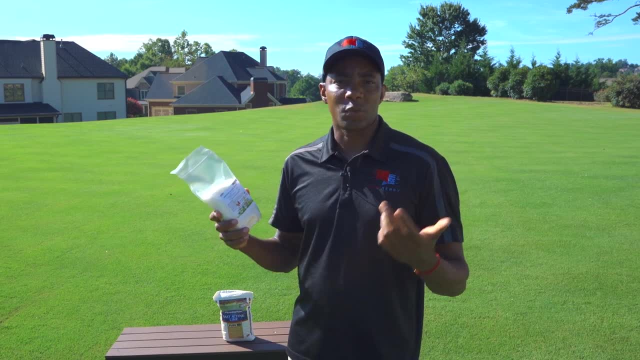 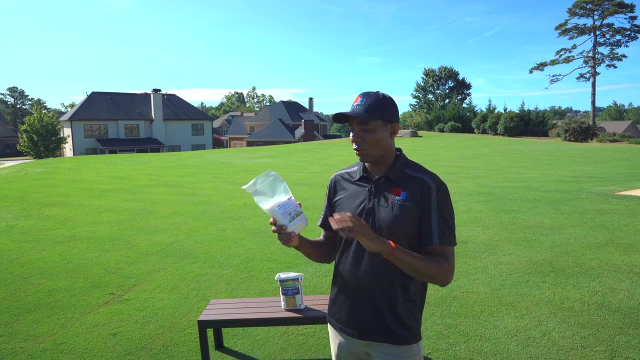 don't. you don't overdo it. you want to put down like a proscape, a 250, you know four or whatever, something like that, and then also apply you know 21 nitrogen on top of that. that would be a little bit excessive. so when you're lowering ph, um just be conscious of you know what you're doing. as far, 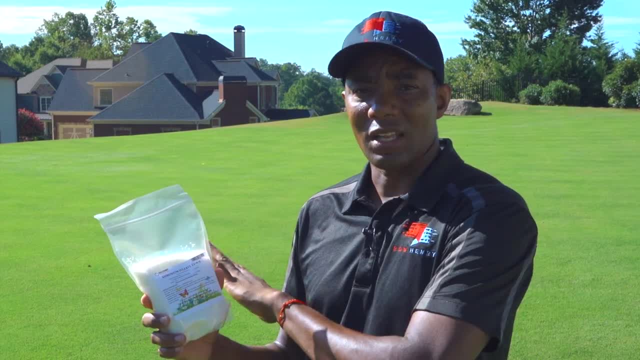 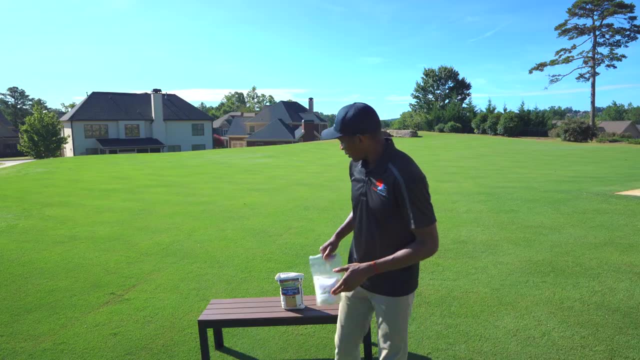 as fertilization and take that into account because, unlike the lime, there typically is a nitrogen component to ammonium sulfate when you're trying to to lower that soil ph. so, guys, i hope you guys found this useful. it's a really quick chat about soil ph, why it's important. it is something 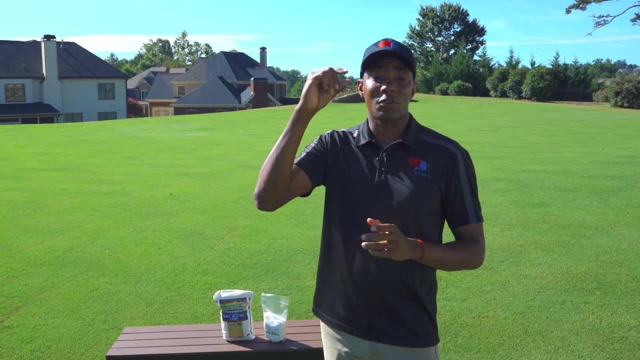 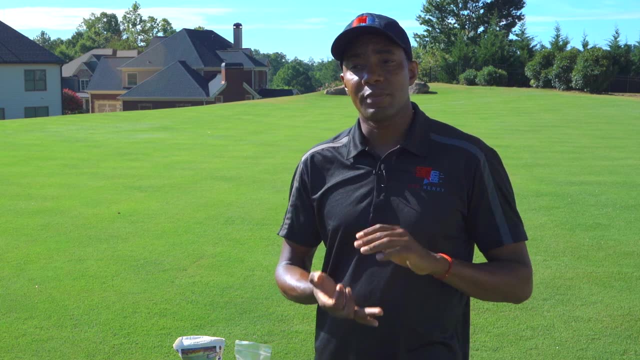 you really should pay attention to in your soil test results. it's really typically the first thing that's listed in your soil test results, because it is really the most important thing to get right, like applying, you know, nitrogen, potassium, phosphorus, you know, putting iron in the lawn.